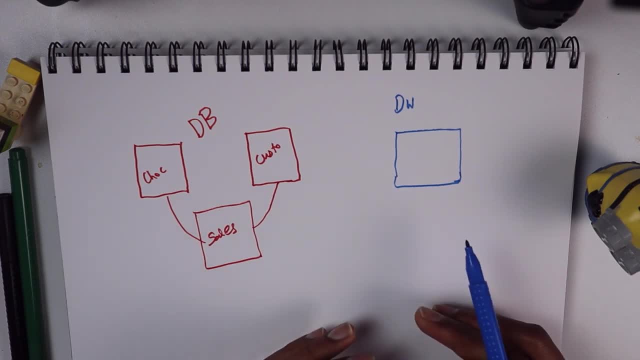 you could then use it and figure out some trends and maybe do some additional analysis and decide on what sort of discounts to offer, what sales promotions to run, etc. so a data warehouse is a special type of a database that is used for reporting purposes. you might think why. 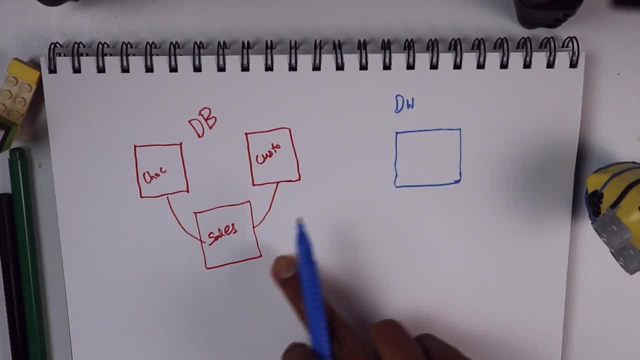 can't we do this kind of thing right here? what is the purpose of having two different things? there is a reason why companies try to make a database and a data warehouse within the database. the purpose is to keep track of the business. so let's say, you drop a particular type of chocolate. 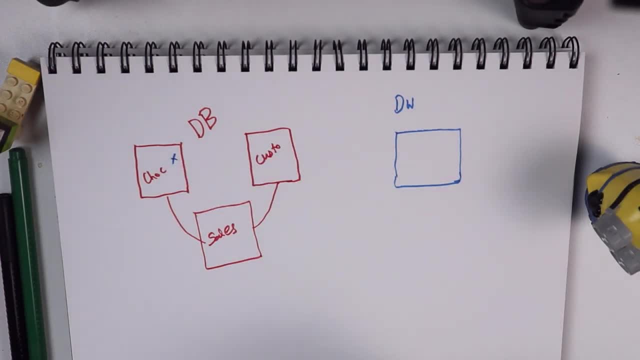 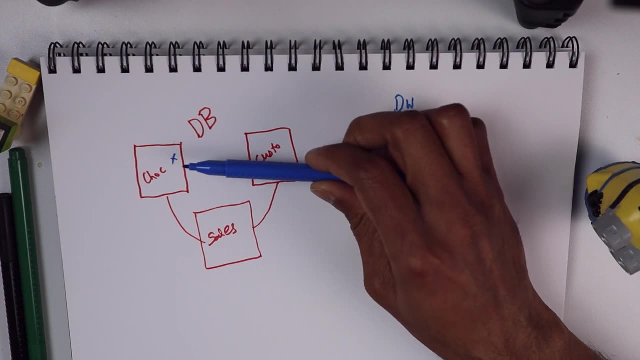 from your database, then you use this as a database. so what you would do is you take a slightly different product line. that chocolate gets deleted from here, then if I want to know how many of those drop chocolates that we have sold in the previous months, it will. 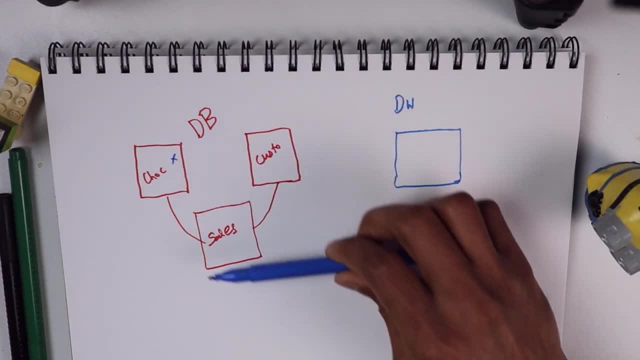 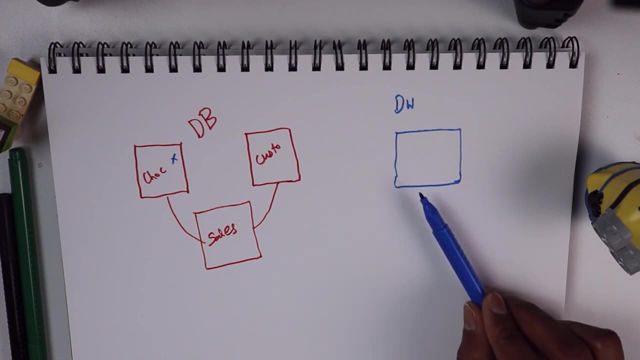 be very tricky to answer that question because that record is no longer there. we are not able to establish the linkage and get the relevant information. for that reason companies use data warehouse. within the data warehouse they periodically archive the data, so all the data from here is taken and then kind of 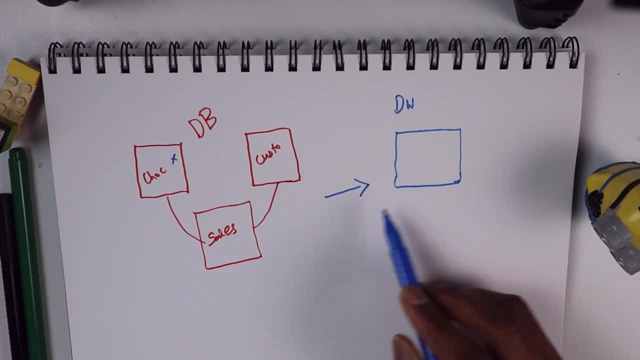 reshaped and moved into the data warehouse on a regular basis and then you can use this, because it is kind of like a historical repository of the data. all the information is stored here. I can ask a question about how many of those dropped chocolates we sold in the year 2019, and we can get the answer from data. 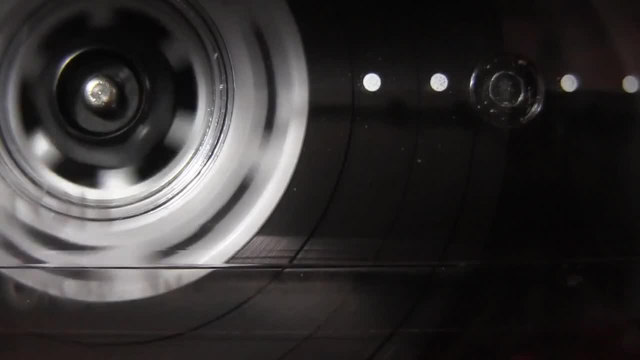 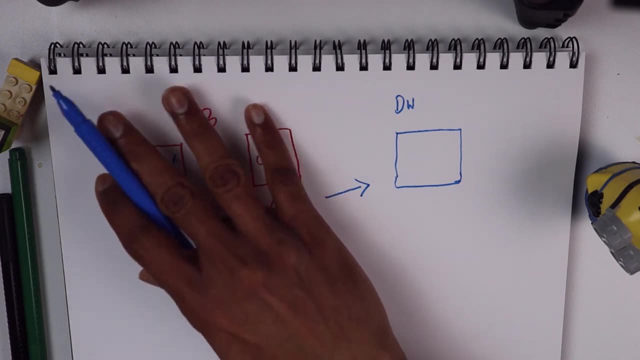 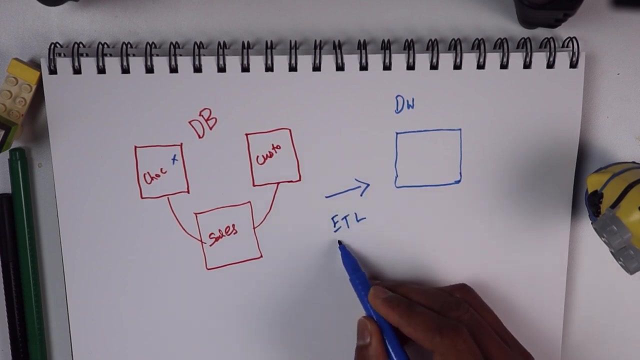 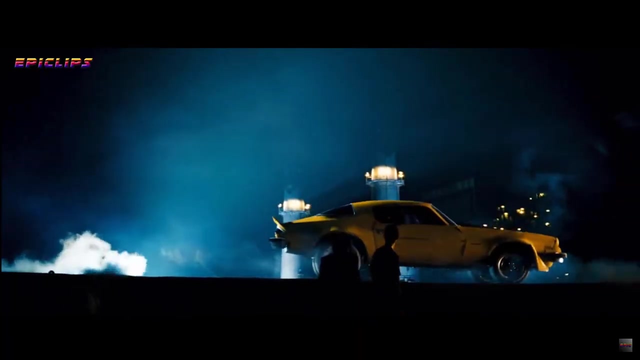 warehouse. one simple way of thinking about data warehouse is it is like a tape recorder that is just recording all the things that happen, this process of taking your database data and then loading it into data warehouse. he is also called as ETL, extract, transform, load- obviously not that kind of transformations. so then, what is a data? 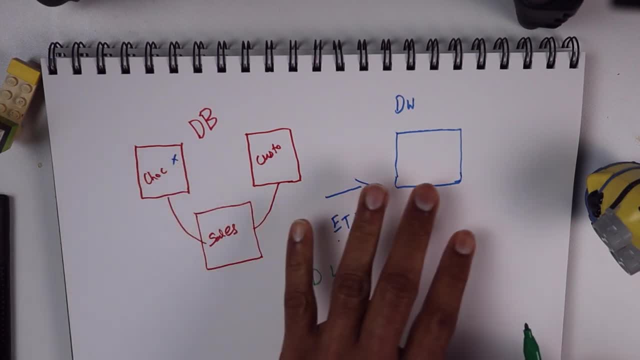 lake DL. within database and data warehouse, the traditional way data is stored is a table. a table is nothing but a bunch of rows and columns, each column explaining one type of data, but sometimes you may have to just store other types of data as well, so a data lake is basically like a 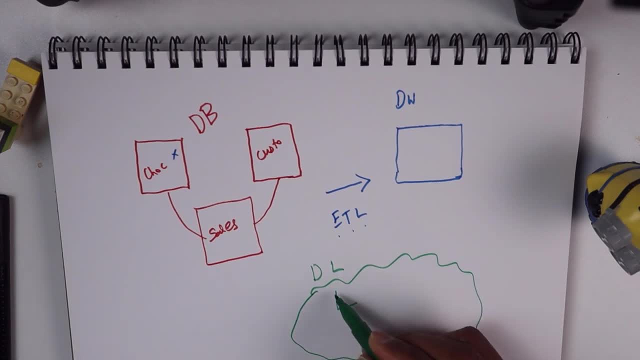 place where you just keep everything. it can contain some of your tables, it can contain some of your files. it can even contain some images and movies. that's just me drawing an image. so you might think: what is the point of data lake? why would you even bother making a data lake? we got all of these things nice and 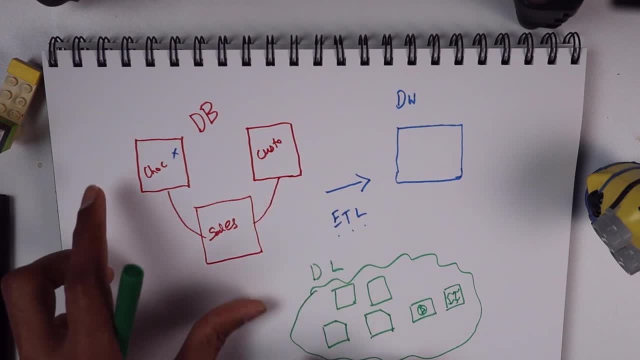 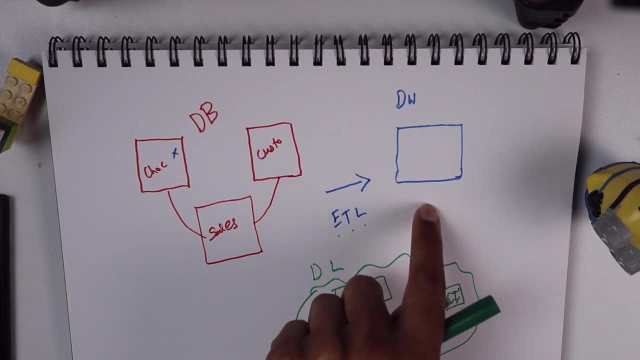 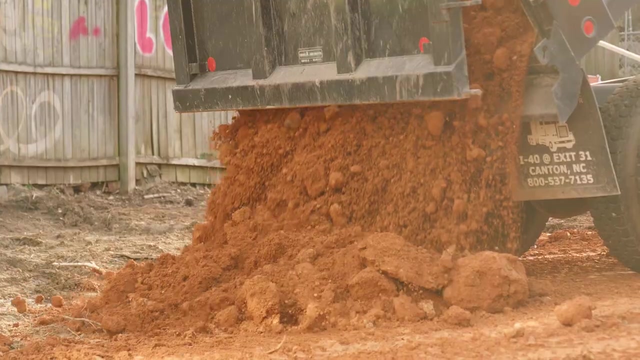 clean here. this is because within a database, you have to design the database so that your business can operate within a warehouse. you have to design the warehouse so that you your reporting needs can be met. but sometimes you don't know what you want. you just want a place, like a dumping ground, where things 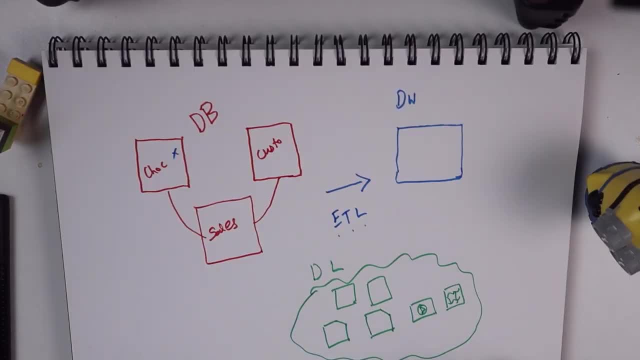 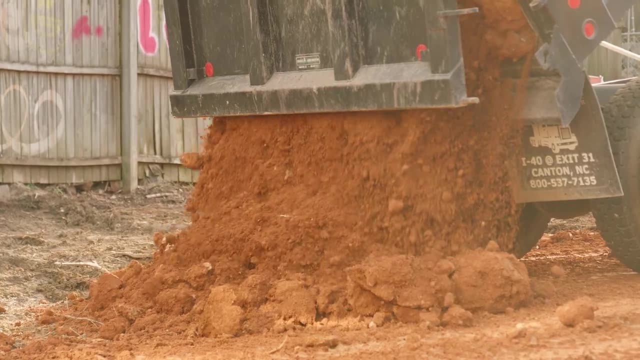 should be kept so that later on you can ask any type of question. so that is where a data lake comes in handy. you here, you just kind of store everything in a semi structured manner. I'm not really saying, like you know, go and dump things, but you will kind of maintain. 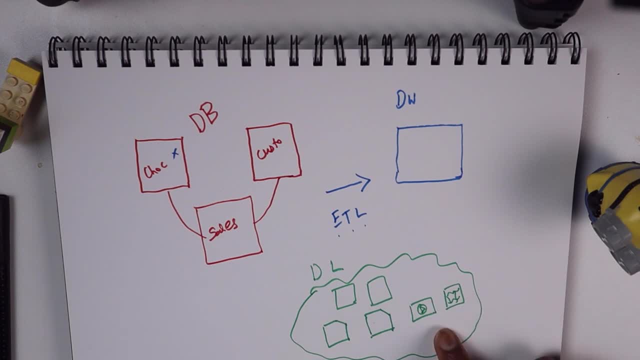 some sort of structure here, so that you could then use either structured approaches, like asking a question and getting an answer, or unstructured approaches, like asking computer to figure out what is going on. this is where all your artificial intelligence, machine learning and other algorithmic type of things will come in. 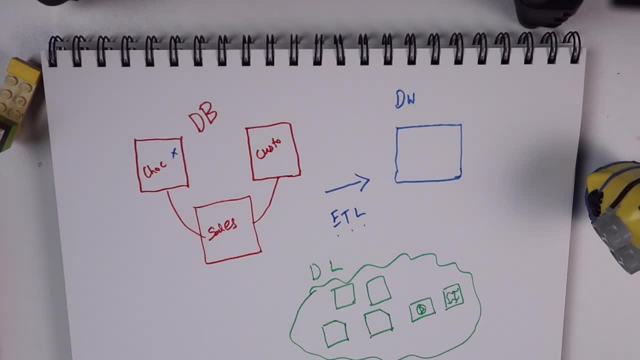 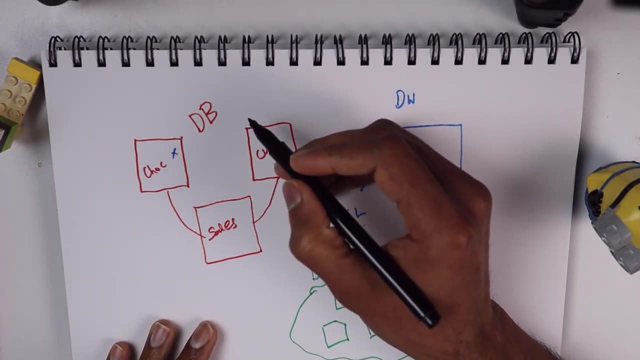 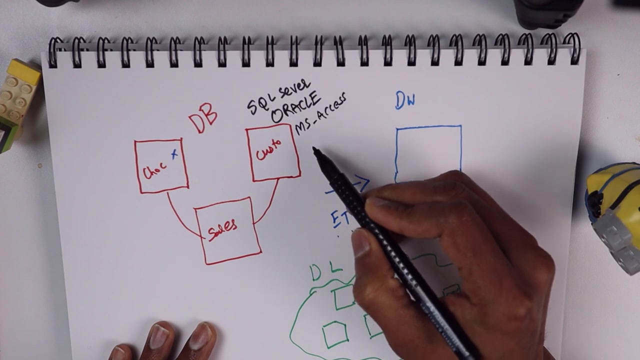 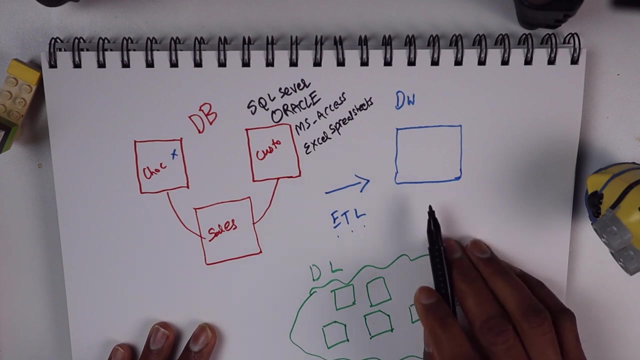 so that is where data lakes come in. so what are some examples of database, data warehouse and data leak us. let's address database. an example database is your SQL server, oracle, MS access or, if you are running a really small business, even Excel spreadsheets. what about a data warehouse? a data warehouse, as I said, is a 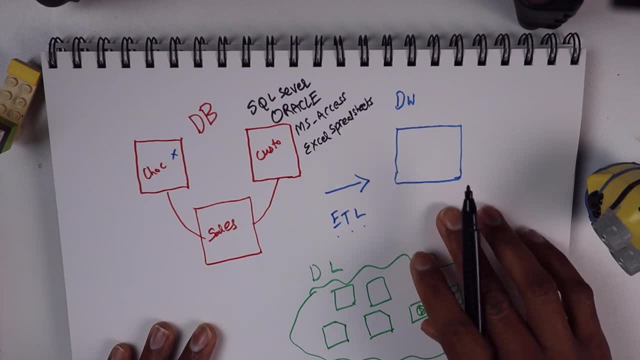 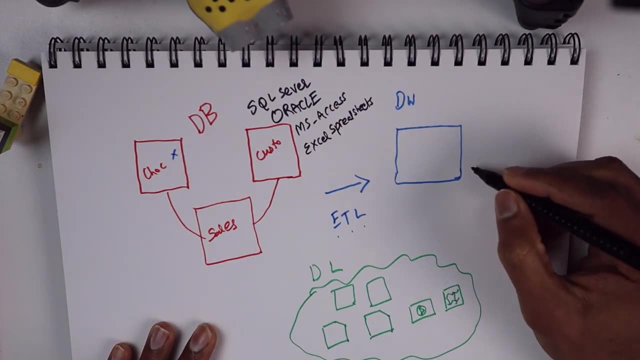 special type of a database, so many companies also use a traditional database. oops, that gave a lot. many companies also use a traditional database like SQL server, but there are also some specialized data warehouse offerings. and then, when it comes to data lake, usually the data lake is maintained online. that 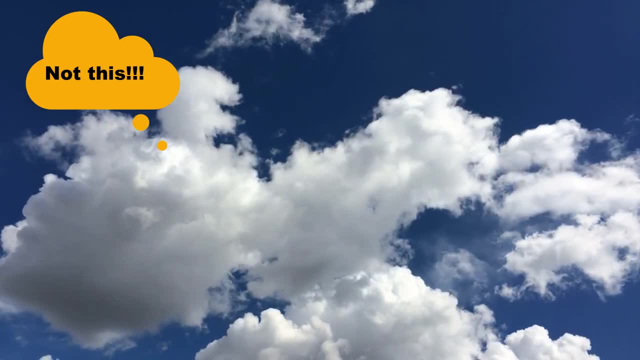 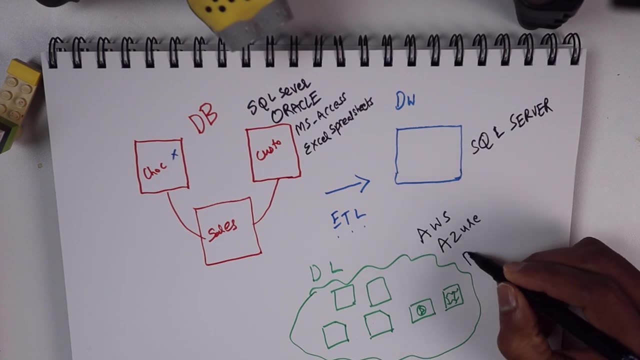 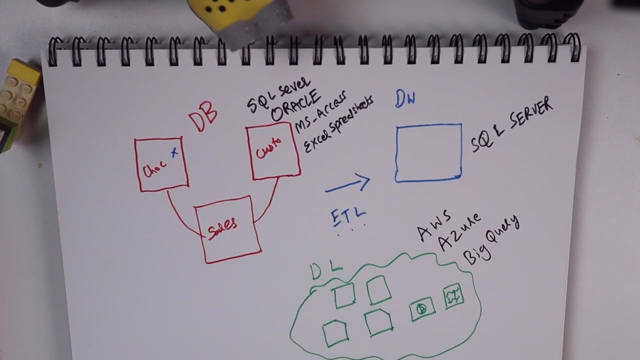 is on the cloud, but sometimes it could be on the premises as well, so some of the standard data lake platforms are your AWS, Microsoft Azure and Google's big query. the next question that you might have is how do we access the information within each of these three things? within a database, the data is